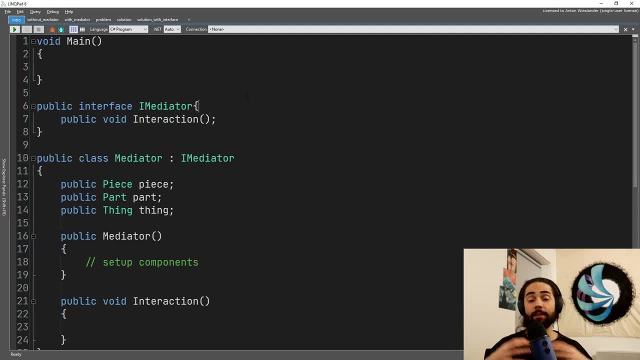 relationship between these objects. So the MediateR aims to take the interaction between the two objects, a cashier and a customer, and centralize that interaction. That centralized interaction is what we're going to refer to as the context. In the context of the checkout, we are going to have a cashier and a customer. In the context of a surgery room, we're going to have a surgeon, we're going to have a surgeon and a patient. The interaction in the 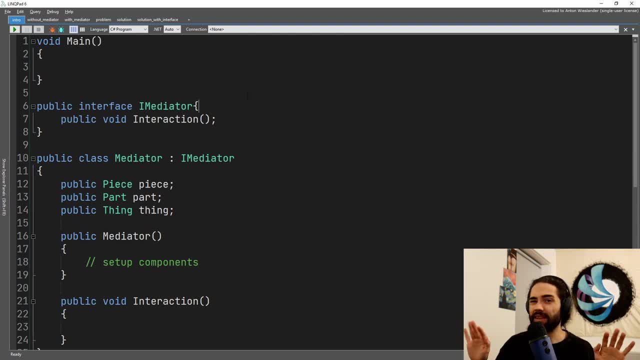 context between the two objects- they're humans but they do play different roles- is going to be different. So remember: the point of MediateR is to centralize interaction between objects. If you're enjoying the video, don't forget to like and subscribe And, as always, if you have any questions, make sure to leave them in the comment section. The implementation detail for this will look something like this: We will have an interface which will describe the iMediator. In our case, the iMediator is the name of the pattern. 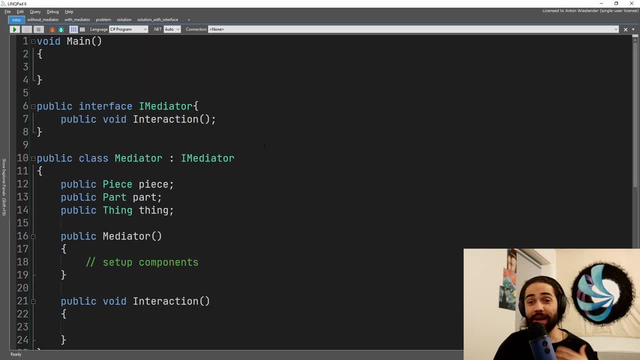 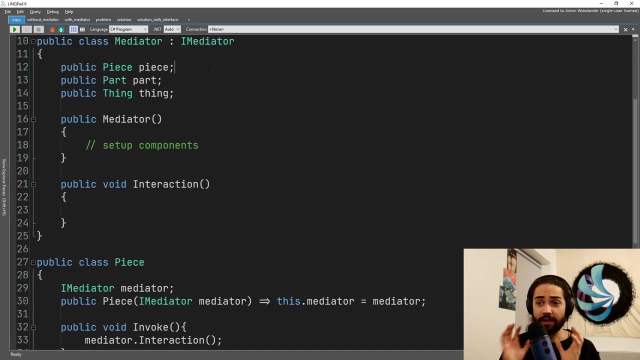 When you're going to be implementing it. don't call it by the pattern name, call it by its intent. Make sure it's descriptive. What is the context in which this is happening? Is it a surgery room? Is it the checkout? Is it a battlefield? What is going on here? Right, In our case, this is just the MediateR. So, within the MediateR, as the centralized context or what can happen, we can have like some pieces, some parts, some 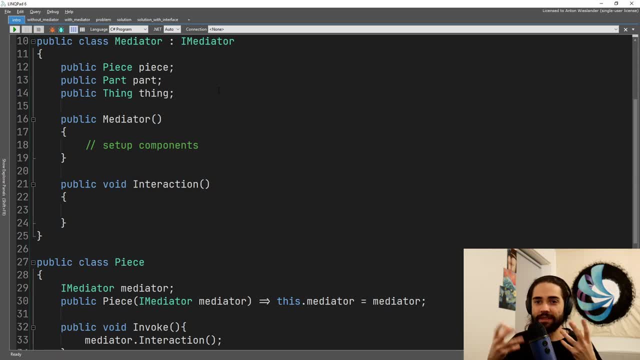 things, essentially the little components that are going to be interacting. those are the humans: that will be the customer, that will be the cashier, that will be the surgeon, the army dude, etc. whatever other profession you can think of. so mediator does not take care of giving each individual role to 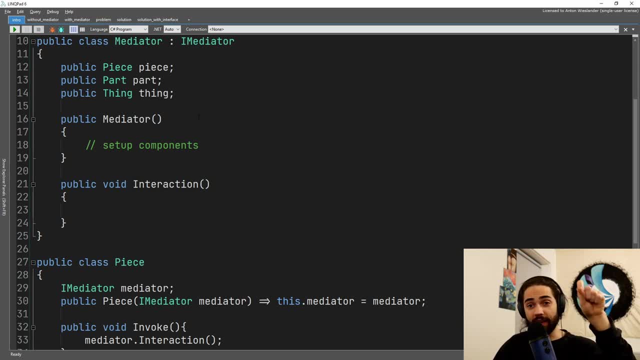 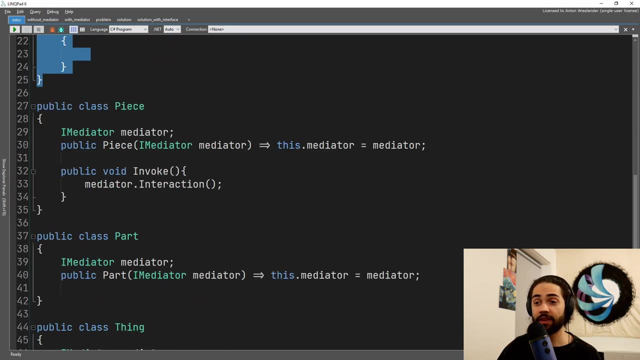 each individual object. okay, so we do not go ahead and give the doctor role to the human in order to make it a, that's that specific role to have those particular functions. so, mediators, main concern is centralizing the interaction between the objects. so this is where the interaction happens. we then 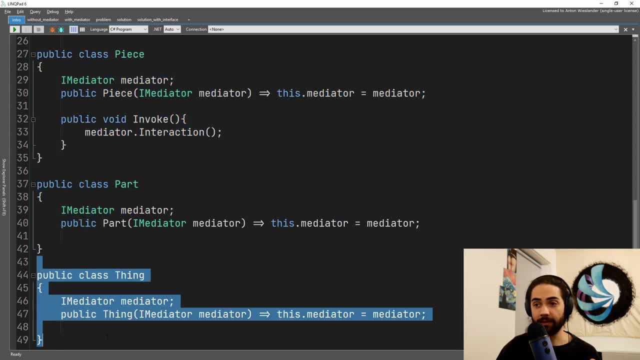 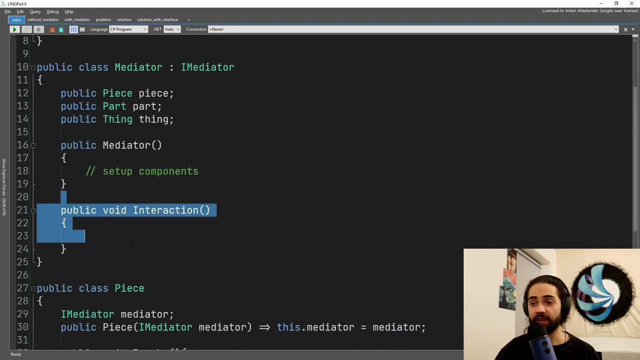 have our particular piece, our part and our thing. each of them receives an instance of the I mediator and whatever interaction they essentially want to invoke on the other ones, they trigger it through the mediator. as soon as the piece invokes the interaction, the interaction will be available to the person who wants to invoke on the object. 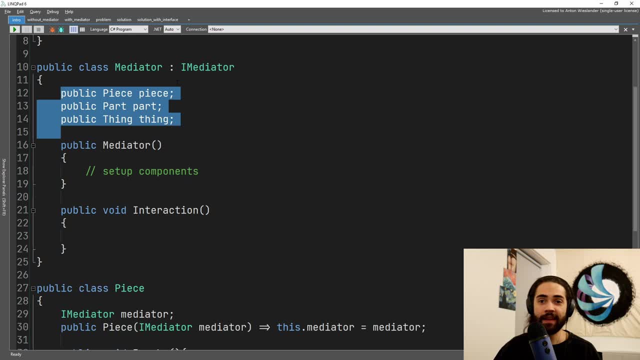 enjoy the video, so that's a special way. by the way, you can make it that specific role to have. those can then act upon the piece, the part or the thing, essentially any component within the mediator. Compared to the mediator library, this is a very concrete implementation. But let's take 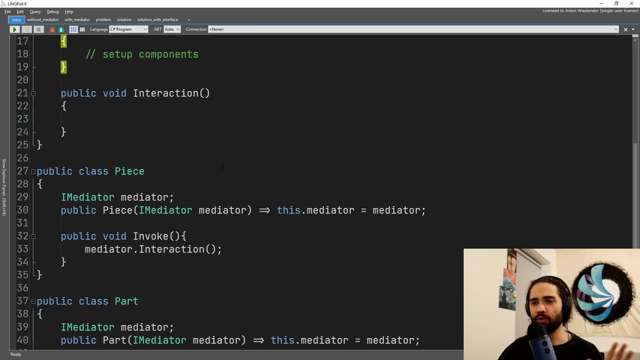 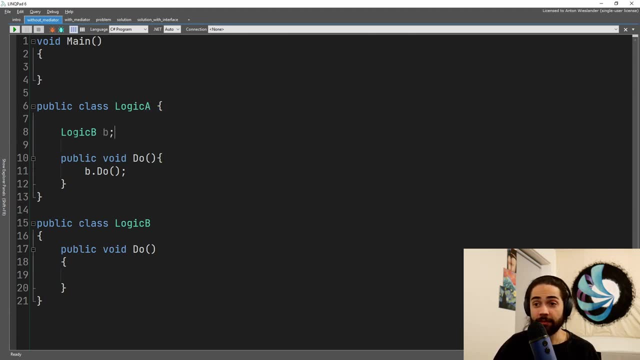 a look at a little bit more of a simpler example if this was a little bit too generic in terms of its names. So, without mediator, we would have logic A, our cashier, and it would have to hold a reference to logic B, which is our customer, And we would have to perform some kind of operation. 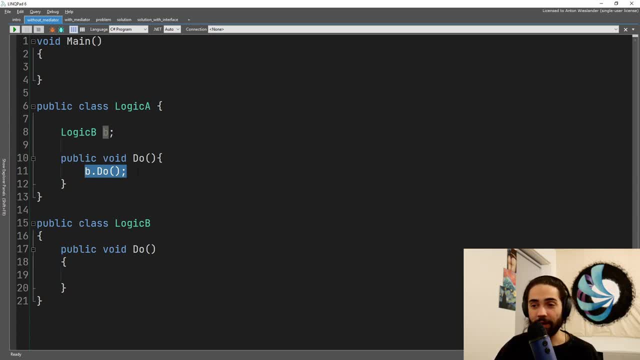 like ask for money and then put a request for money into the customer, and then the customer would then have to trigger its own function, And you can see how both of these would have to have a reference to each other and trigger each other's functions in succession. Now enter the mediator. 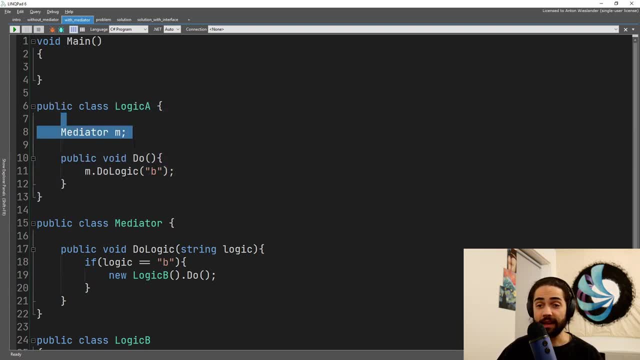 Now logic A: the doctor contains mediator, Which is the surgery room or a patient. I don't know wherever a doctor room, right, Wherever you're going to prescribe the medicine on here, he's going to check your health or temperature. 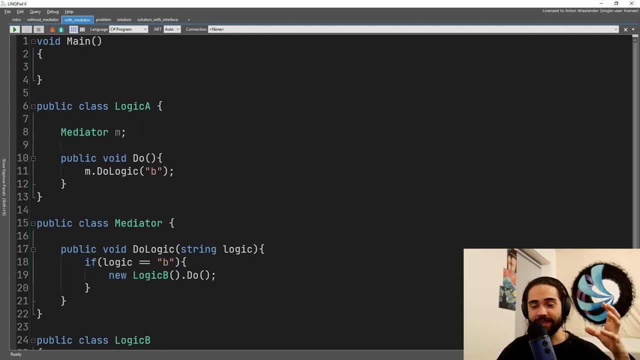 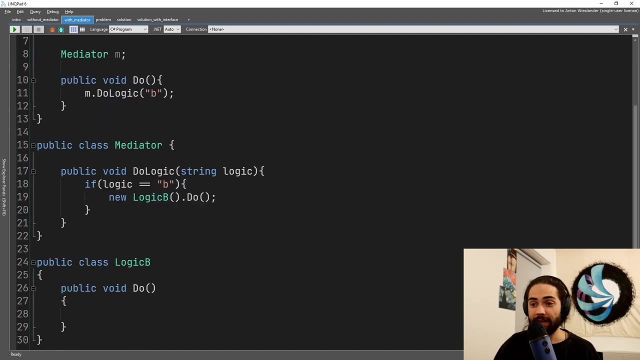 whatever doctor room. okay, So mediator is the doctor room. So we have the doctor, he's in the doctor room And as soon as, as long as we have the patient in the doctor's room, we can dynamically trigger whatever logic we want. We can check his pulse, check his breathing, and you know. 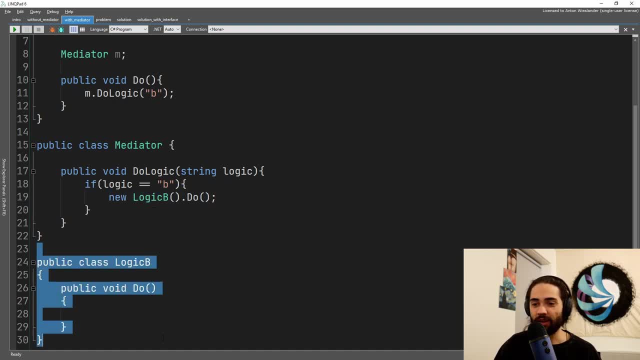 when he, you know, check your breathing. it's like on the, on the customer or on the patient. you gotta go say ah, and then the guy goes ah, and then you go breathe deeply and go, all right, so yeah. 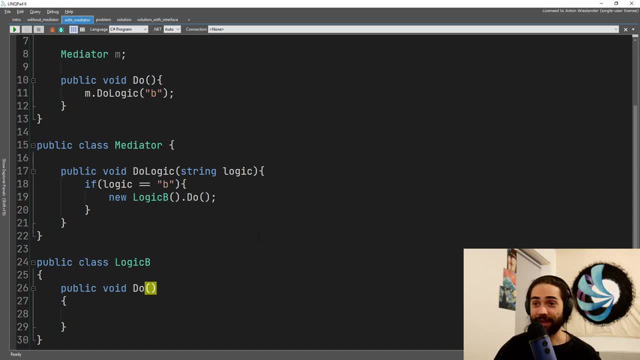 issues command and then logic B- the patient performs the command. right, This all happens within the medical room or doctor's room, okay, And what happens in the doctor's room stays in the doctor's room, okay. Now, going a little bit further into the problem, maybe a more. 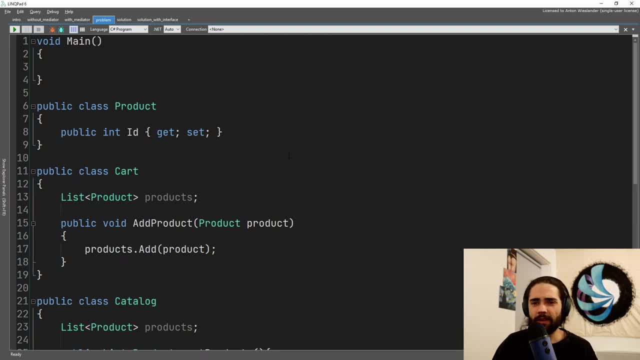 a little world example. I still wouldn't consider this very well thought out example because generally, if you're watching my tutorials, this does tend to be more on the back end. but this problem is more on the front end, And on the back end we have mediator and that is. 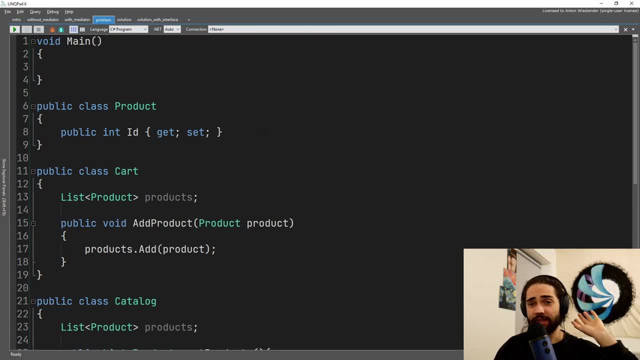 very decoupled, very message-based implementation. It's very generic and it's very easy to use. So I highly recommend to go check out that library. But in this example we have a product, an object, and then we have a product, and then we have a product, and then we have a product and then we have. 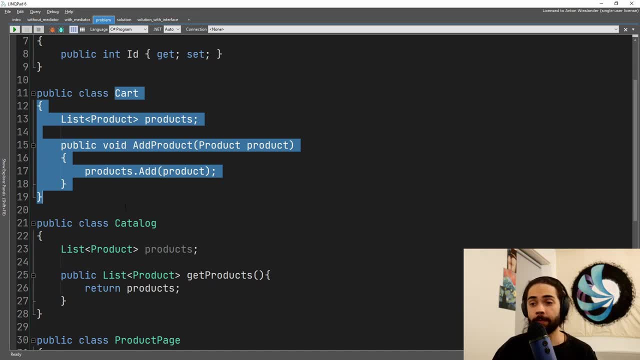 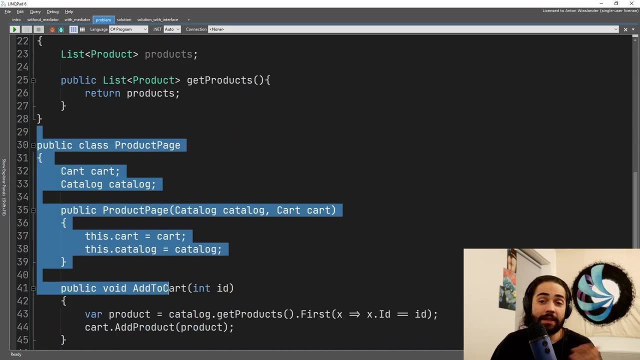 a cart, So again somewhere where we can put products. and then we have a catalog, So the things that we can purchase, So we can grab things from the catalog and we can put them in our cart. This has to happen somewhere, So we put that catalog and that cart behind the product page. 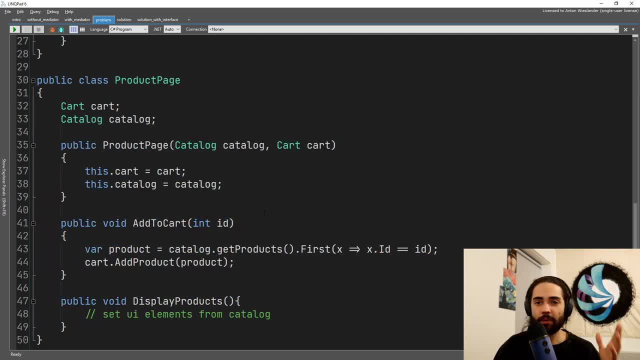 and they kind of live here, They kind of live in the product page. So the product page now relies on having catalog and cart. So there is now essentially heavy dependency here between the objects and the interaction between the objects. So let's say 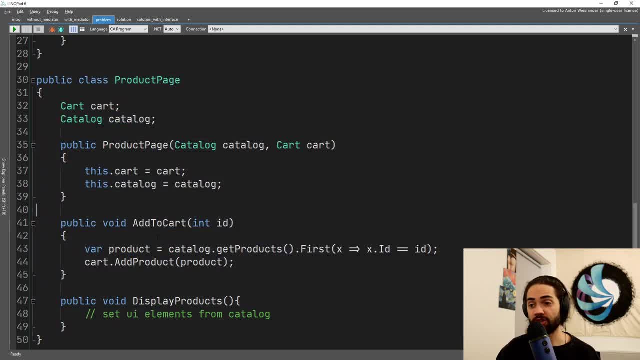 we want to add a product to cart on our product page. This scripts the interaction where we get a product from a catalog and we put it in our cart. This logic is no longer reusable anywhere within our shop. I don't know if you visited much online shops, but you are able to. 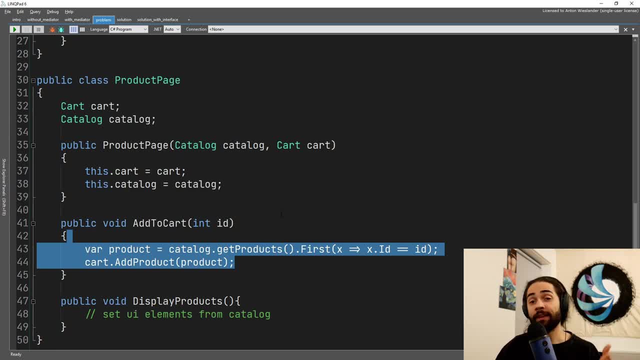 add products from multiple places within the website. right On the front page just add to cart. or then you visit the actual product with the big description and you find a button there to add to cart. or you can press the plus button, minus button to increase or decrease. 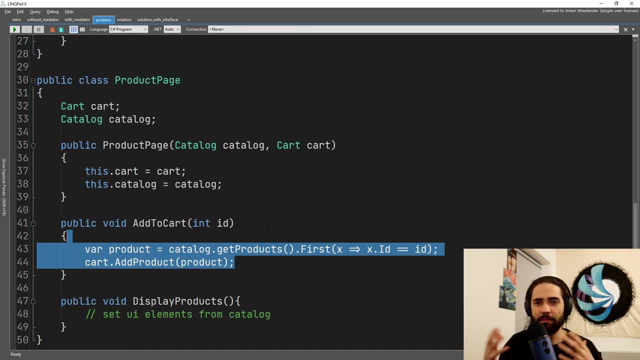 quantity, So you can add and remove products in many different ways, from many different places, And also the way that we display the products. we have to have a reference to the catalog And this is the catalog which is within our shop. We do not have the option of importing. 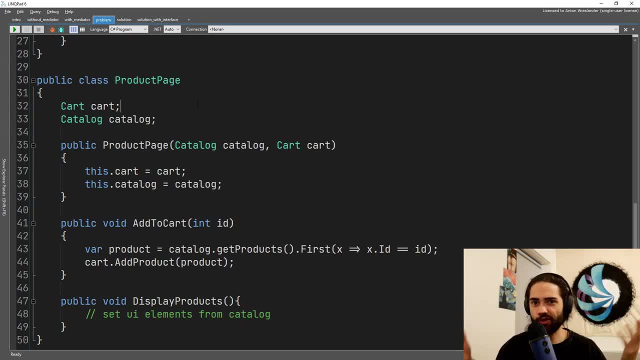 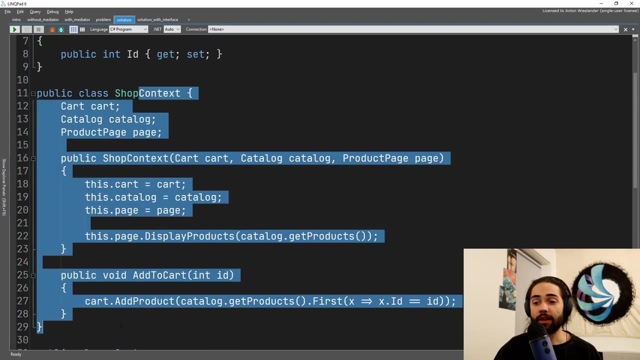 products from somewhere else and injecting them into our shop, right The way that YouTube does with Teespring, and for some reason They don't allow third-party integrations. I don't want to use trust issues, whatever, So enter the solution. We still have a product, but now we are centralizing the shop context. 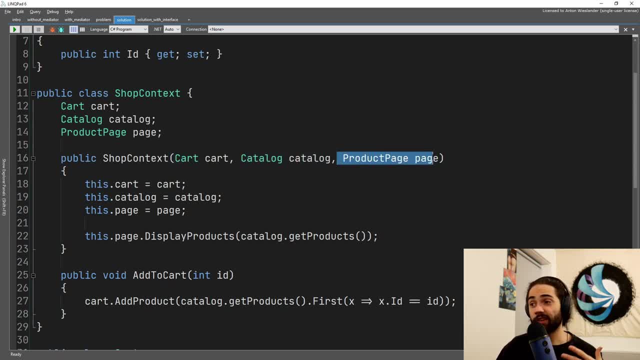 The shop context is the thing that holds the cart, the catalog, the product page. It is the thing that pulls everything together, like the Spider-Man and the scene where he's like holding the train or whatever. So, yeah, it has all of those things and then it goes ahead and also injects the 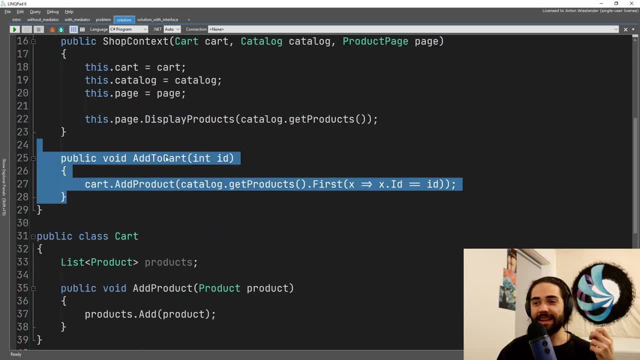 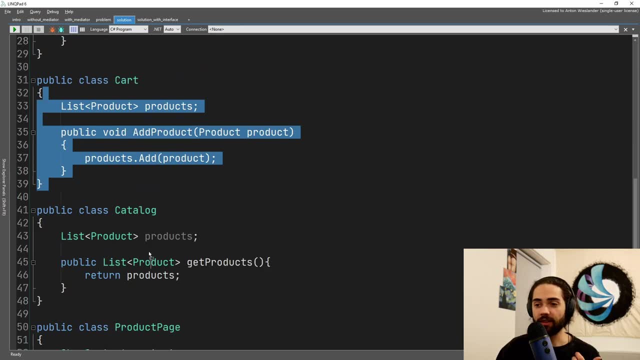 product into the product page And it essentially contains a add to cart function which is like a proxy function to the add to cart. The cart is the same, The catalog is the same. It's not real implementations here, It's just to. 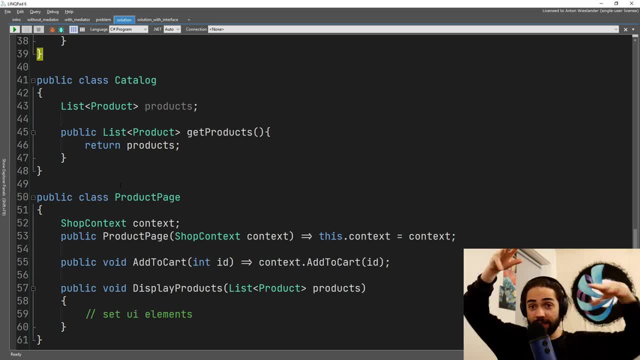 illustrate the idea. So, as long as you can imagine that we have these components and you are just centralizing the interaction between those components, Do not try to go back to your code and force things into this pattern. Just understand that at some point the interaction between your 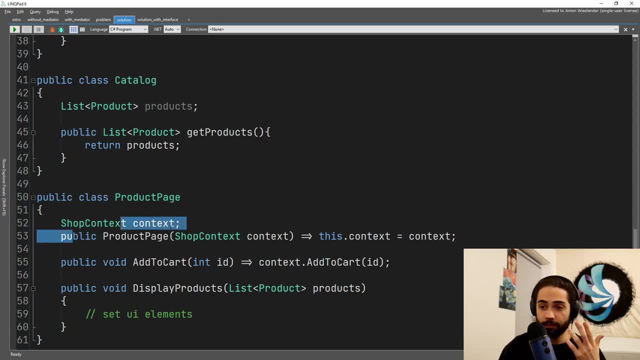 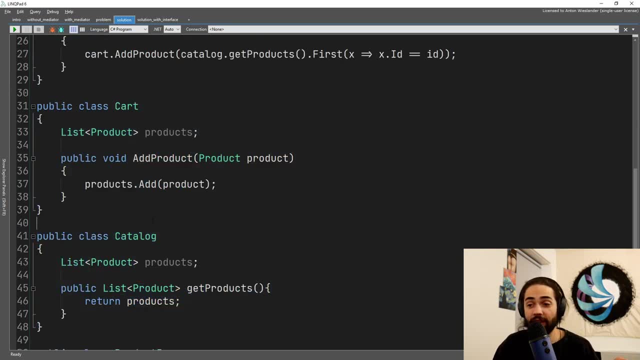 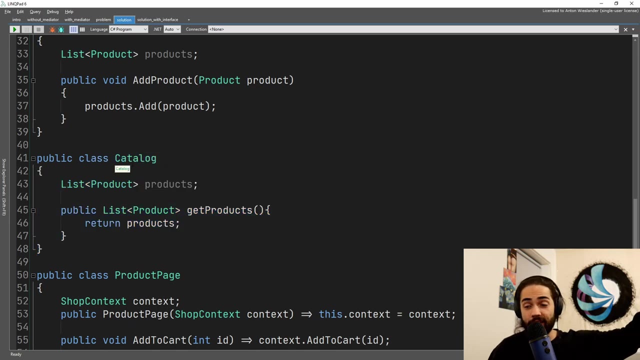 components is going to look muddled, But right now what's going to happen is we just receive a shop context. If the catalog or the cart can do something along the lines of we at the checkout, we basically purchased the last product, a catalog will say it just ran out of a product and it will broadcast it to the shop context. 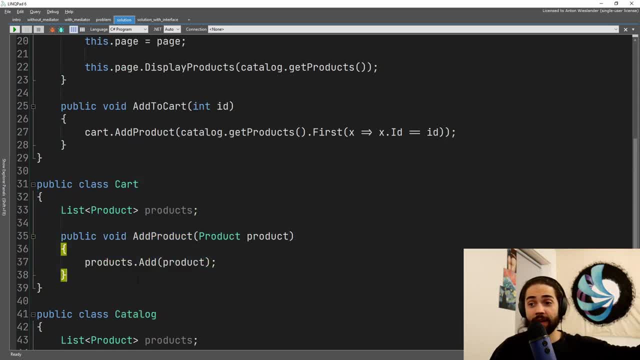 The shop context, can then go into each individual cart and clear out that product because we no longer have it. And in the shops we assume that we sort of have infinite amounts of products or you get a lock on the product. Anyway, that's implementation detail. The point is that the 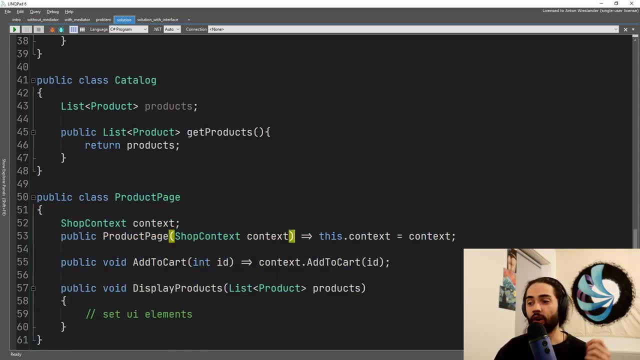 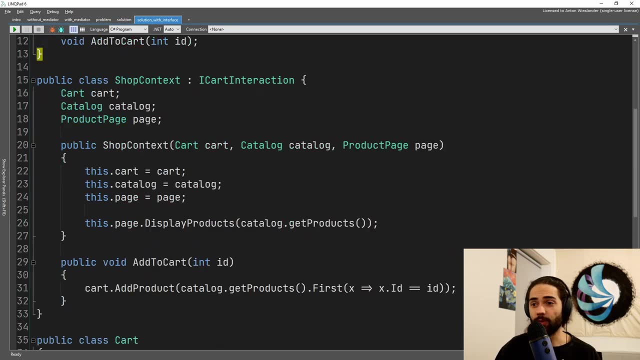 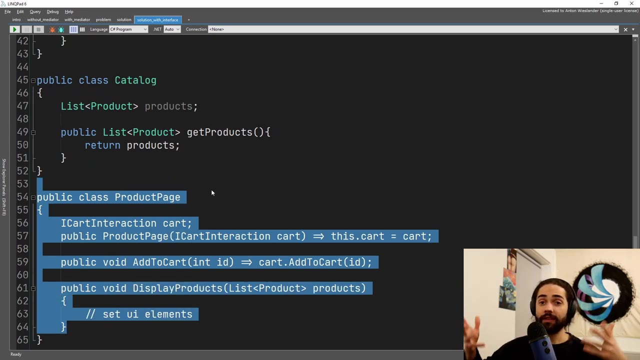 product page has now access to the shop context and on there it will be able to add the cart. We can take this a step further and forget about a shop context. We can hide it behind an interface like cart interaction. So we can either hide the cart behind an interface or then later upgrade to. 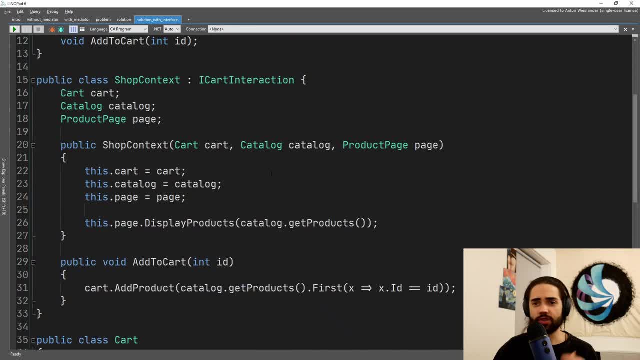 a shop context. And again, if you are struggling to imagine where to use this pattern, think of the facade pattern. If you haven't watched that video, I recommend you go watch it. We essentially have many components. They know how to talk to each other And what we do with facade. 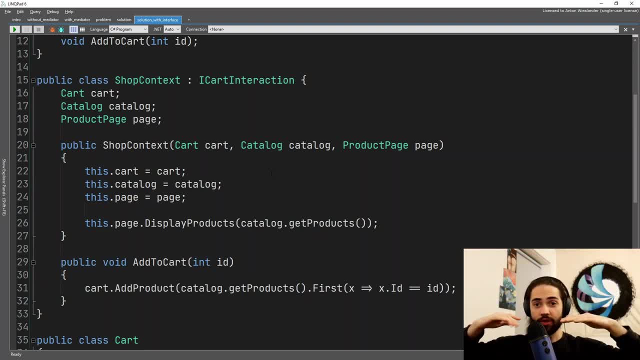 we essentially put that interaction in a box, we push it down and then we can access the facade as like a very, very convenient thing to use to interact with the subsystem. If we take a look at the subsystem, the way that it interacts is we essentially have a. 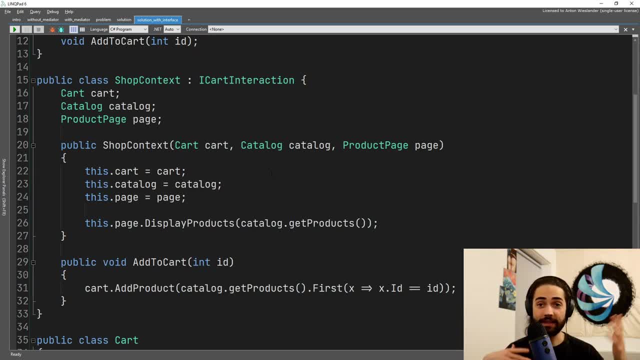 spider web with dependencies going in every direction. There is no structure there. Mediator is more or less meant to bring structure to that. It will take the spider web between the components. So you have like 10 components and the lines are going from all of those components.